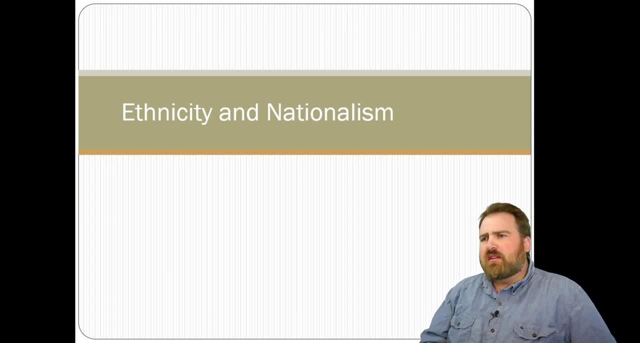 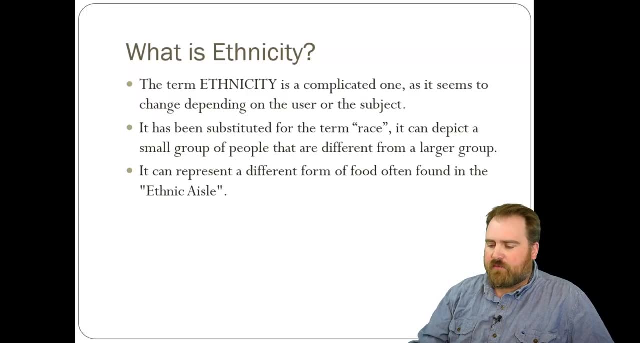 on race and culture. So let's go ahead and hop into it. So we have to sort of figure out what is ethnicity? Essentially, ethnicity is this: it's a complicated term that oftentimes gets misused. Oftentimes it's sort of substituted for the term race. 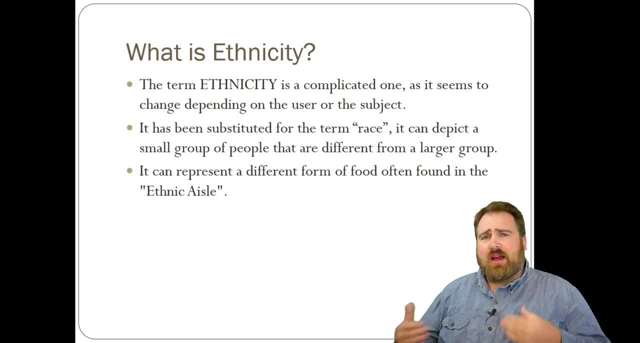 And that is absolutely not how it's supposed to be. right, Race and ethnicity are two totally different subjects, And so we have to understand what's going on with these terms. Race deals specifically with biology, right And sort of the expression of those genes. right, Ethnicity. 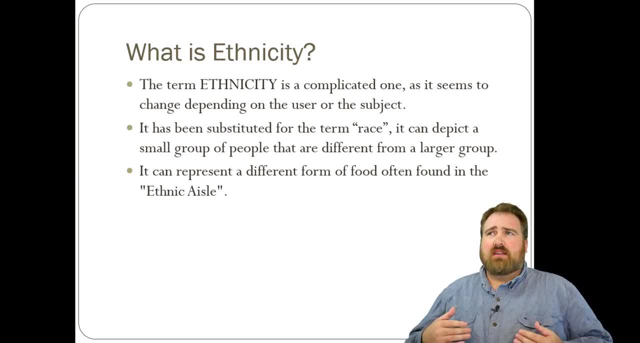 is about culture, Right, And so sometimes they get intermixed, but we shouldn't do that, okay, And we'll talk about why that's the case. So it gets used in a lot of different ways that it shouldn't, So hopefully, 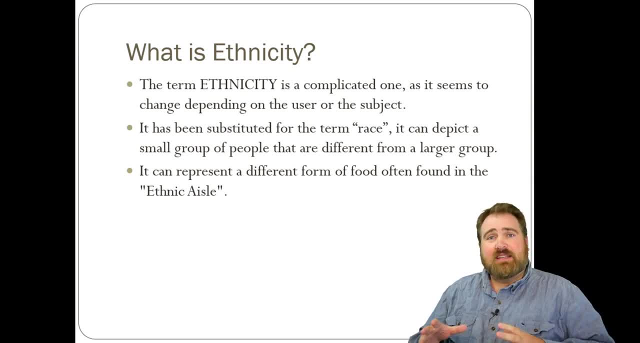 you'll learn. you know just about that. You know the fact that you know this is how it should be properly used. Also, a lot of times people just find ethnic in stores, right, You know, in the ethnic aisle. 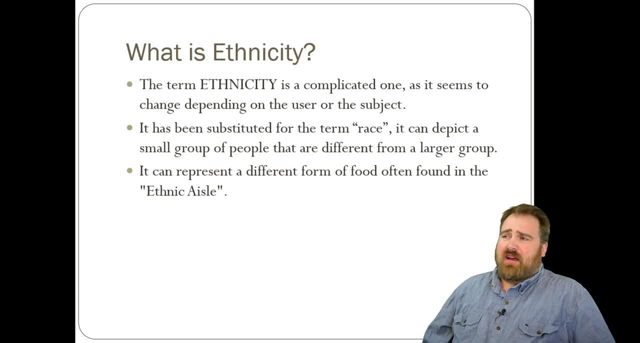 of the grocery store, which is where you'll find, you know, different types of foods from all over the world, But we set aside this term to sort of say- and I hate using this word and I've brought this up before- is to use the term exotic. 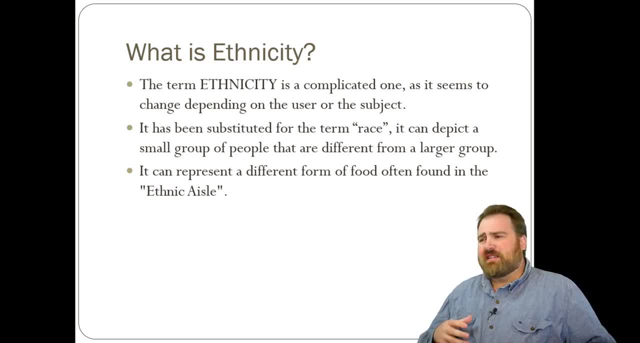 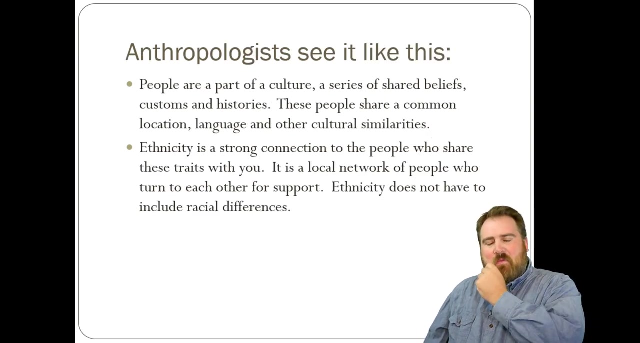 So oftentimes things that are seen as different, as exotic, can also sometimes be misused as the term, like ethnic. So you know, that's kind of toss that out right there. So yeah, this term has a lot of different connotations to it. Now anthropologists understand that. 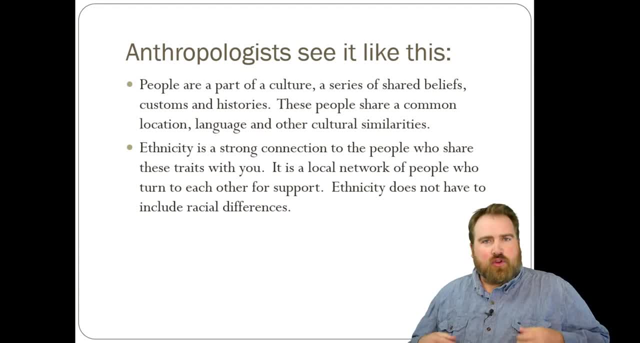 ethnicity is really just another term for culture, Okay, And it's all about the fact that we have, we see, people that that share a common history, common language, common geographical location- And again, this is really important for concepts of ethnicity- and have these similar traits. 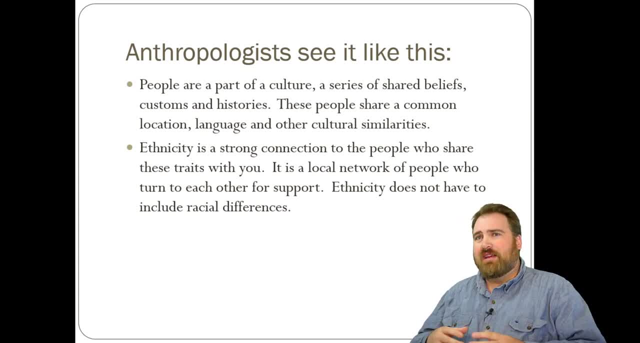 Right. So when we talk about culture, when we talk about what our culture is, where we are in the, What constructs a culture, the norms and values and mental maps and all of that stuff, right, These are all things that draw us together. 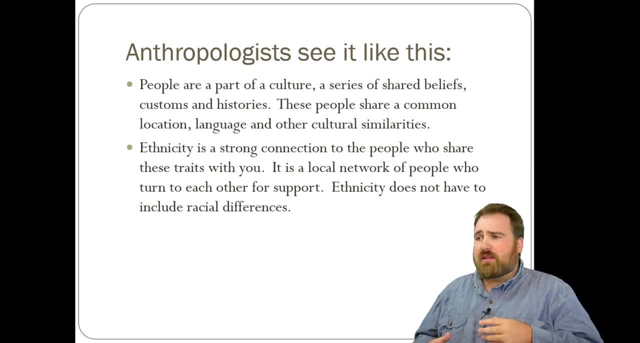 We all have similar. We might not always agree, right, Because in culture we are oftentimes contesting what other people might say or believe in, but it's still there, right, And geography has a big part of this as well. 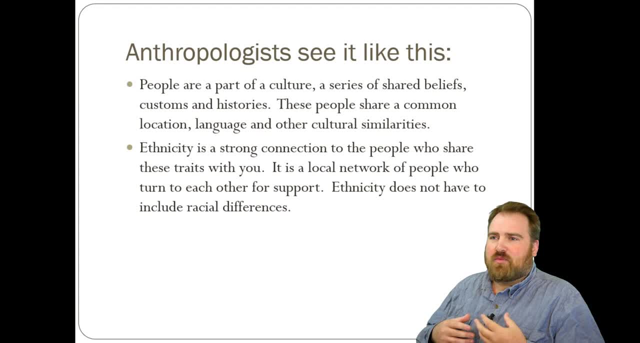 So, really, you know, anthropologists, when we look at ethnicity, we're talking about culture. When we're doing, when we're studying a population, we're doing ethnographic studies right. So this term is connected to culture and to these different ideas. 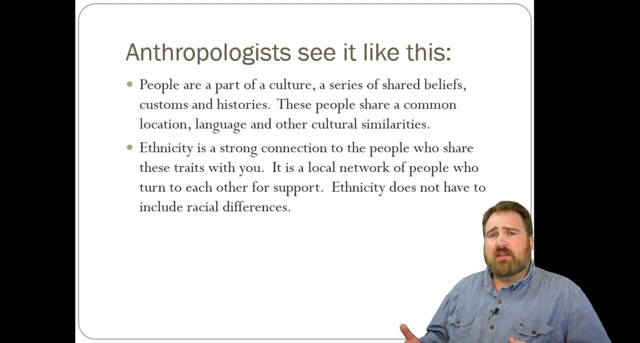 So when we talk about ethnic groups, We're really talking about cultural groups, but it goes somewhere further than that, because when we talk about ethnic groups, we oftentimes talk about groups that might be a part of a larger nation, so they might be part of a country, or they might be nationless, right? 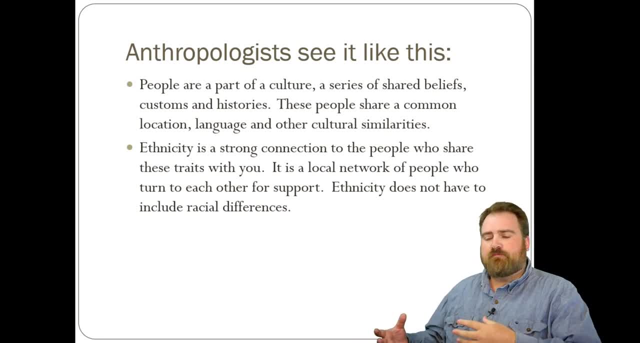 So they might not actually have a country to call their own, and we're going to be talking about some of that as well. So anthropologists understand that ethnicity is really just another term for culture and that all of the things that we define as culture get sort of fit into this ethnographic study that has all of these things combined, along with geography. 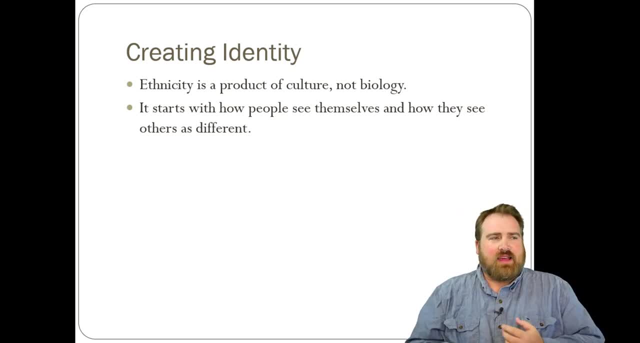 So when we're talking about ethnicity, we're talking about it being a product of culture And not biology. Now, what do I mean by that? Well, again, this comes back to this concept of race. So you can be racially something. 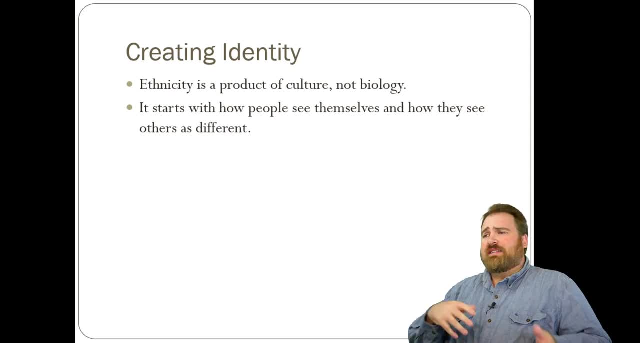 You can be white or black or Latinx or whatever, but you can belong to different ethnicities. right, You can belong to different cultures, So race can fit into different cultures, But a culture itself does not have to be exclusively represented by a particular race. 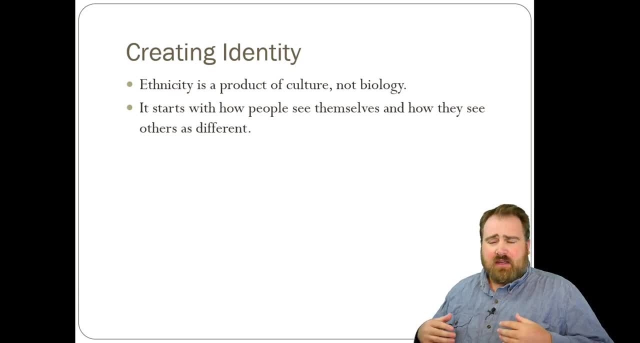 So you can have all kinds of different races being included into this concept of culture and of identity. So again, it's about culture. It's about you know how people. It's about how people see themselves. It's how they see themselves as different from other people. 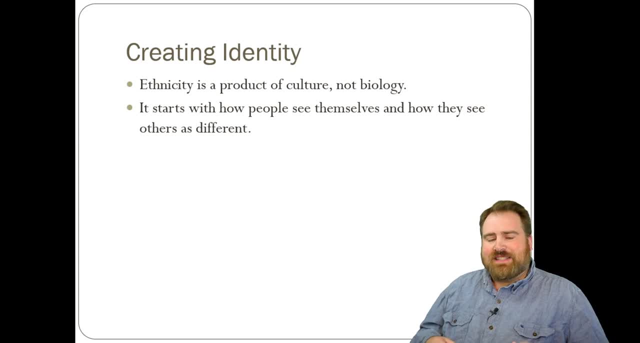 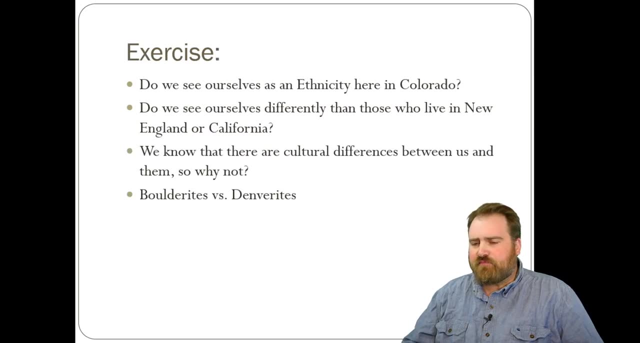 Okay, It's making those distinctions from one community to the next And it's what brings people together. So first off, I want to just take an opportunity to do like a quick exercise and kind of discuss some of these concepts, And then what I'll have you do is discuss one or two of these various subjects in the discussion boards. 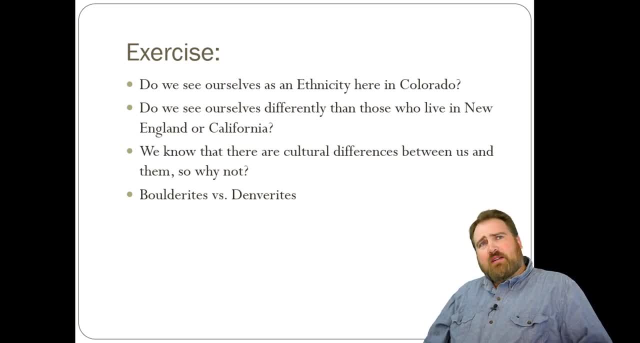 So you know, we've kind of talked a little bit about this earlier in the semester, but I'm going to bring it up again. You know, do we see ourselves as an ethnicity in Colorado? Most people are going to say no just because a lot of people don't recognize that as the case. 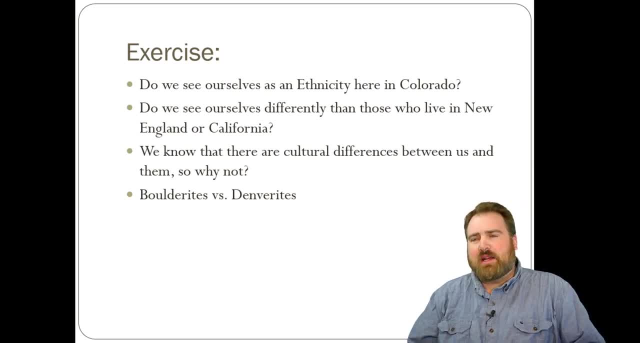 But when it comes down to distinguishing ourselves from, say, another part of the country, say like California or Texas or New England, well, that changes things a little bit, mostly because when you grow up in an area you learn the dialogue right. 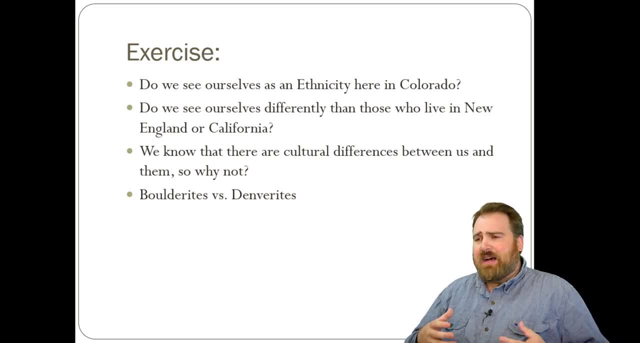 You understand that. let's say, in Colorado we have certain terms that we use When we're talking in language about how we represent ourselves. So if we talk about the front range or the western slope or we talk about hitting some, pow right. 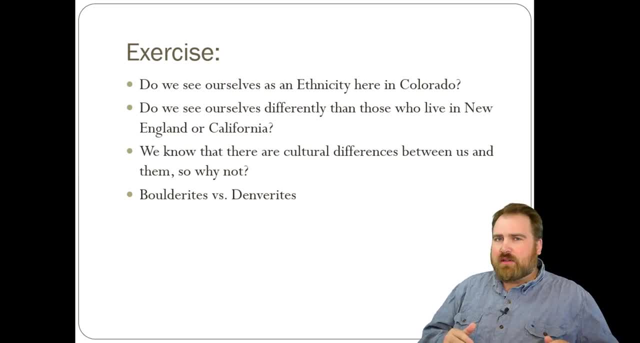 If you're from Florida, pow means something very, very different, you know, than it does here in Colorado, Because we're talking about going up into the slopes and hitting some powder right And going skiing or snowboarding or tubing or whatever I was going to say: floats your boat. 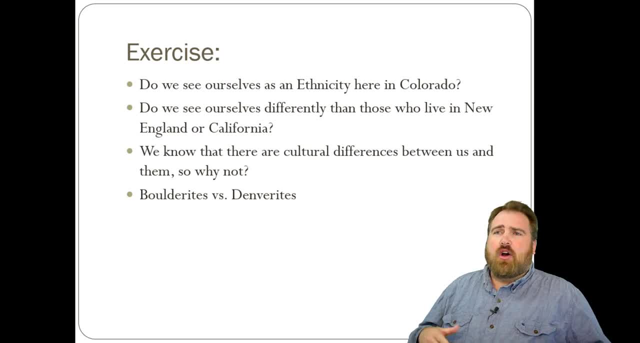 But you know, really gets you down the hill. So there's that right And there's going to be terms that if we were to be in Florida, if we were to go to New England or to California, that we might hear something that we don't understand. 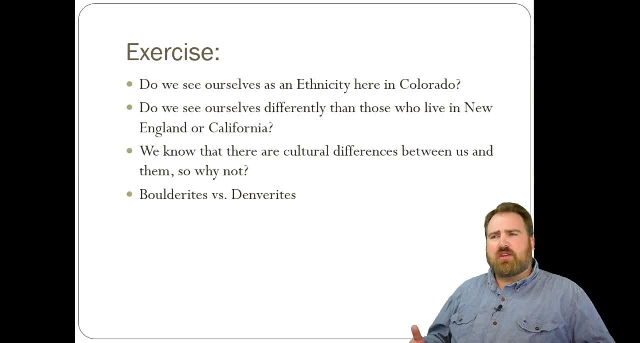 It's like: what does that mean? You know, that word that you just used, you know it might mean something to you and it might mean something completely different to me, And that can be kind of a big part of cultural identity. 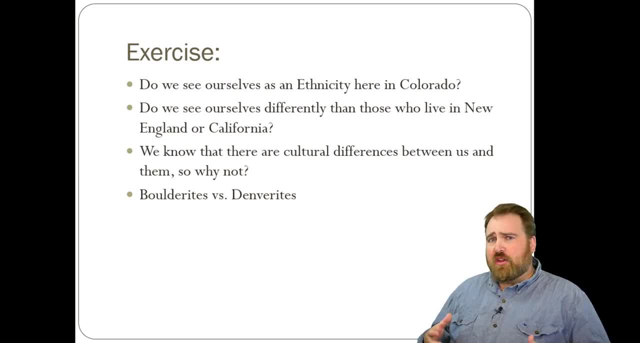 You know how do we, How do we use the language. We for the most part all speak English, But that English can change right If you talk to someone who's from Boston or New York. you know that dialect, that change in how that English is presented can be pretty comprehensive and pretty distinctive. 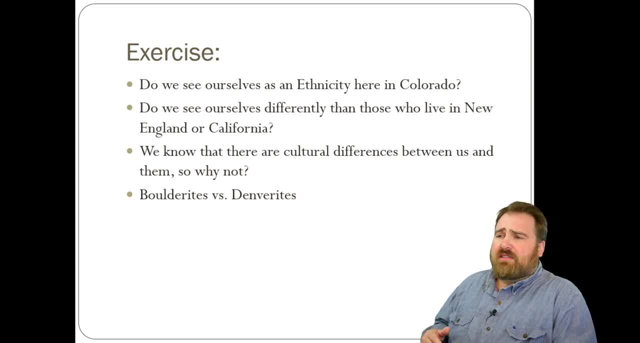 To the point where, you know, I've talked to people coming out of like New York, New Jersey or other places around the country where I mean it was kind of hard to understand what they were talking about. I know we're both talking English, but how things are presented or pronounced can be enough that yeah, there is that difference. 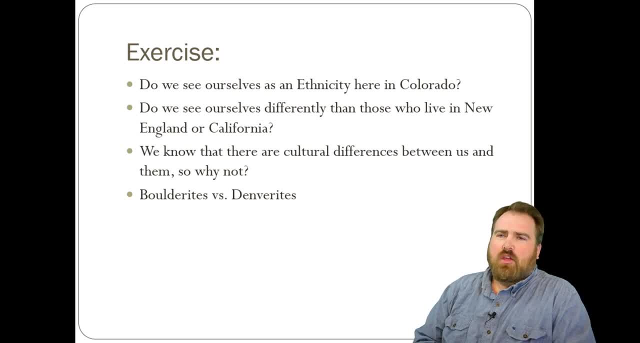 That is, there is that difference in language. So you know, we've got these differences. You know, is it enough, right? Is it enough to say that there is something different between us, You know? and then we can also take it further down, to like Denver versus Boulder. 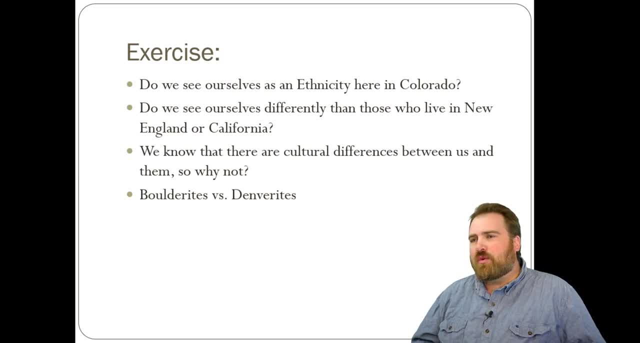 Okay, Now the question is: is there an ethnic difference between Denver and Boulder? And this is kind of a stretch, You know, I put this in here because I think it makes for an interesting conversation, And if we were in class we could have a very interesting conversation about this. 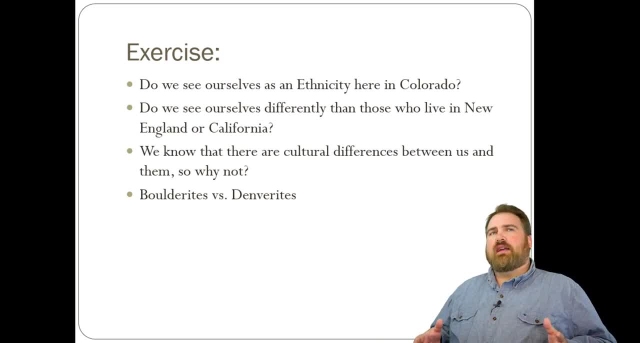 But I'll just kind of toss it out there for now and have you think about it. You know, here's the thing when it comes to Denver and Boulder, And this is an issue where even Colorado's identity is changing, And so it's changing some of the local identities as well. 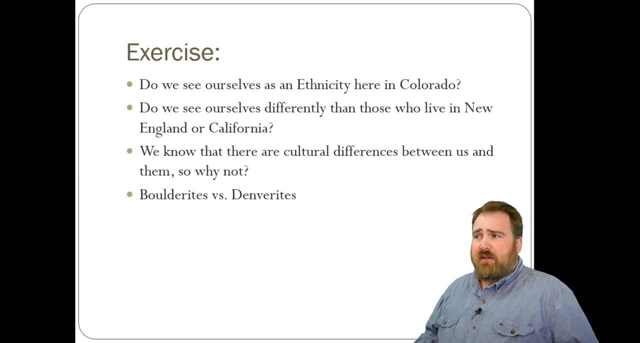 If we were to go back 20,, 30 years And further, the differences between, say, Denver and Boulder were actually much more distinct. Okay, There were some very different cultural ideals in these two towns, And the same could be said for, like, Colorado Springs, right. 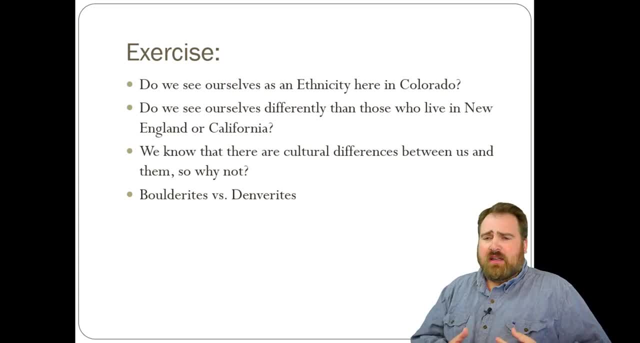 Colorado Springs has a very different sort of structure around the people that live there, Oftentimes because, well, there's a military base And then you've got, You've got the Air Force Academy down there. So the folks that live there have different backgrounds and have different jobs. 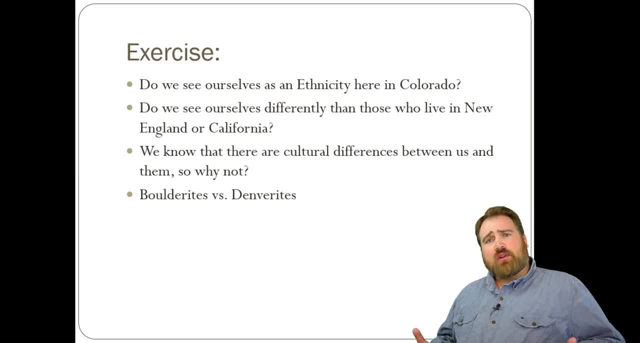 And well, yeah, their culture is going to be structured differently. But what we see here in Colorado right now is we've had such an influx of people coming into the state. You know they're talking. Let's see, I've heard over the last few years that, on average, 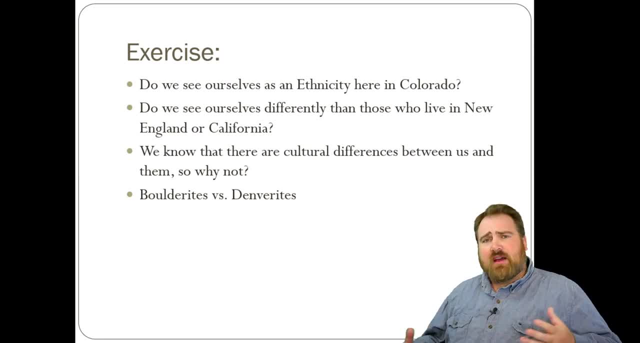 per year. Denver is growing by about 100,000 people, right People moving into the Denver metro area, And that's a lot. That is a lot of people, But what that does is it brings in a whole bunch of different cultures, different histories, different backgrounds. 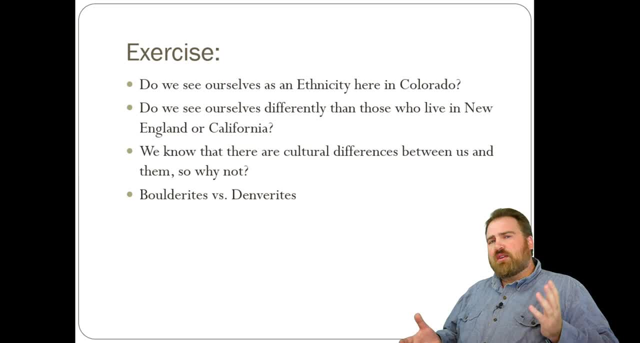 And well, it creates some interesting questions. you know, about identity, That you know sort of this native Coloradan identity which we've, you know, oftentimes flaunted, you know, especially because you get those bumper stickers, you know, on the back of that Subaru, right, that says native on it, right. 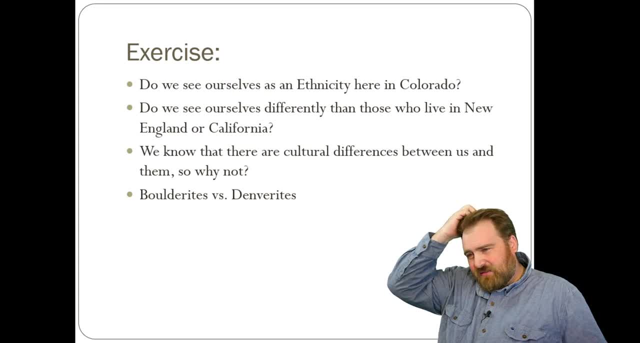 You're a native Coloradan, Well, you know it's turning into something a little bit different than that. We're not really that native anymore because we've had so many people move here, Because, yeah, Colorado's, It's pretty cool. 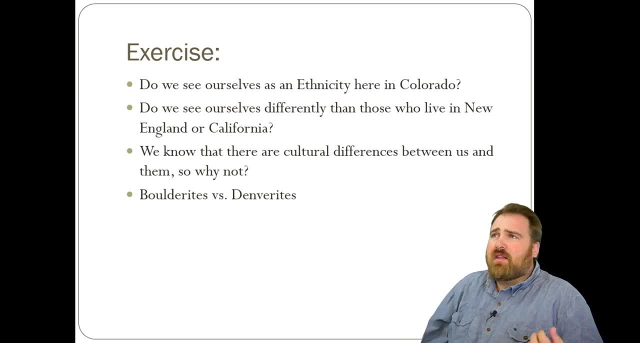 It's a great state So we've had a lot of people moving here, So our identity is changing. So when you have large metropolitan areas like Denver and Boulder and Colorado Springs, as people are moving into them, that historical component isn't necessarily shared as much, right? 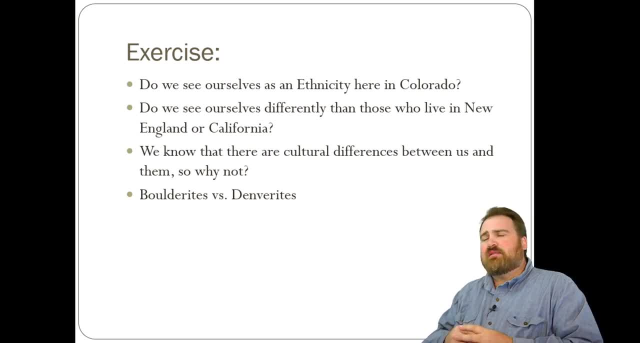 So it creates more of a, More of a generic background. So, and within a few generations, if we had say, people stop moving here for whatever reason, within a few generations that identity would probably become more solidified. As you know, if we have less people coming in, you know, it has a chance to sort of come. 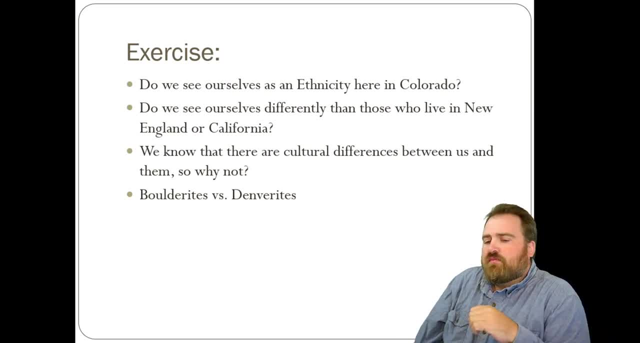 Together and solidify into something. So you know, when we look at these different ideas around, like cities, if we go to smaller cities, well that's a different story. So if we're talking about towns, or you know villages or you know small cities, then there very may well be like an ethnic identity. 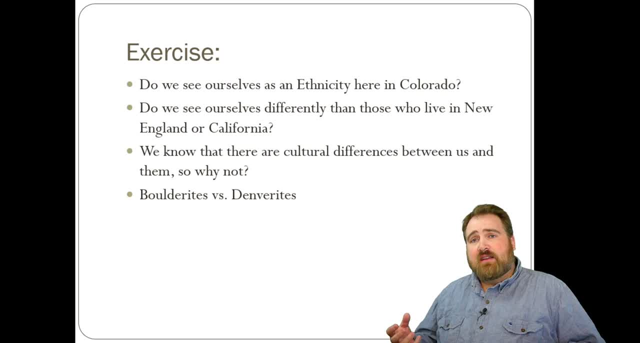 That is a part of that small community And a lot of times it has to do with the fact that you know the people that live in these towns. you know if there isn't a lot of growth or if there isn't a lot of loss and it stays for the most part the same, well, that identity is going to stay there. 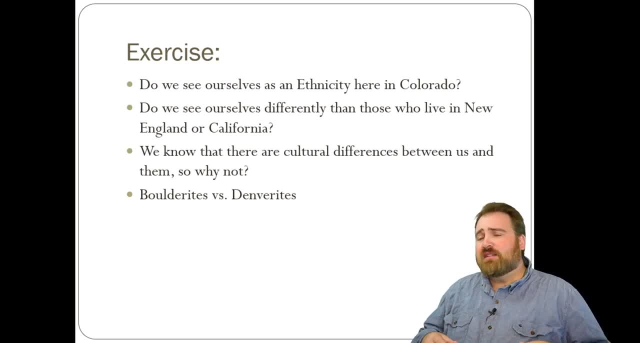 You know the shared history and the shared language and shared jobs and traits and values You know, Become more and more sort of solidified and so that you might have some very distinct identities versus some other town that might be nearby or, you know, say across the state. you know, if we were to compare, say like Fort Lupton versus Cortez, Colorado, right, these are two distinct communities. 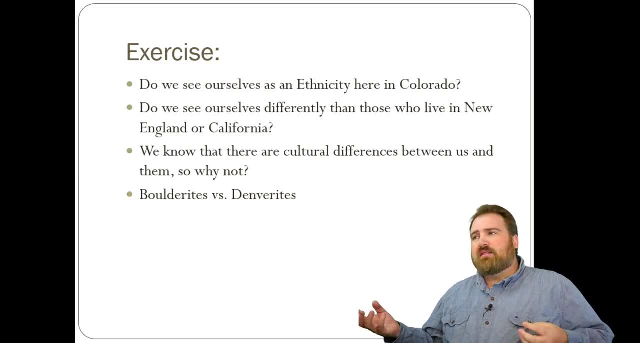 There might be some similarities, but there are going to also be some very There might be some very distinct differences, not only because of geographical location, but because of shared history. right, What happens in Cortez might not be relevant to what happens in Fort Lupton. 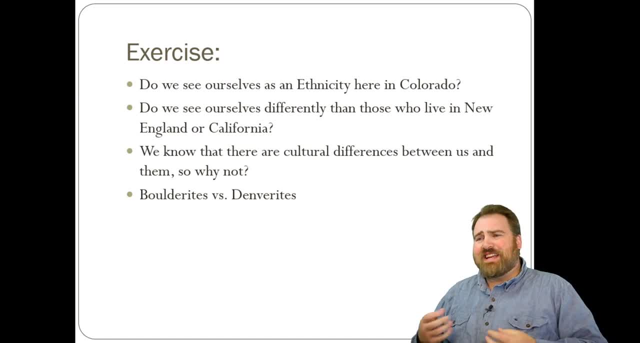 So yeah, so you could have some more distinct ideas about culture and about identity, And certainly within other towns if we go on to like the reservation. So we've got two reservations, Reservations in the state of Colorado: We have the Ute Mountain tribe and we have the Southern Ute. 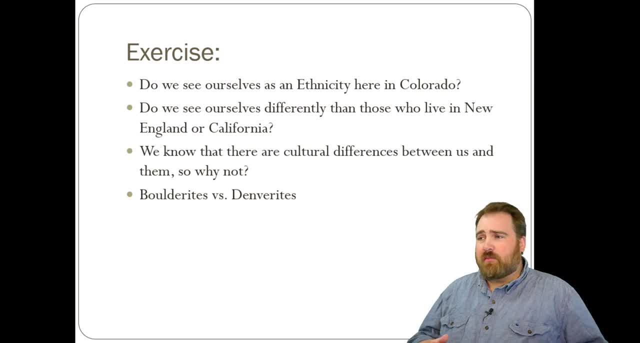 And they are very distinct, right from the traditional Colorado identity. We have Native American groups that have distinct identities, And so we have these different groups, different towns that can be distinct from each other and culturally different. So, yeah, so if we're talking about ethnicity, you know we oftentimes have a tendency as Americans to generalize because of our identity as American right. 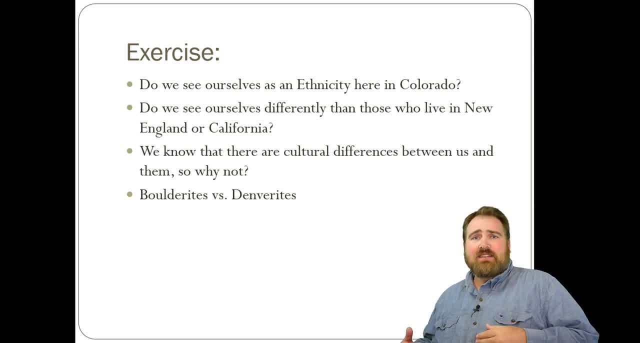 Oftentimes we're American first and Coloradan second, right, And so you know we might pick that national identity first, And we're going to be talking about some of that later on In the lecture series. So I want you to think about how these different concepts you know are coming through and take an idea.